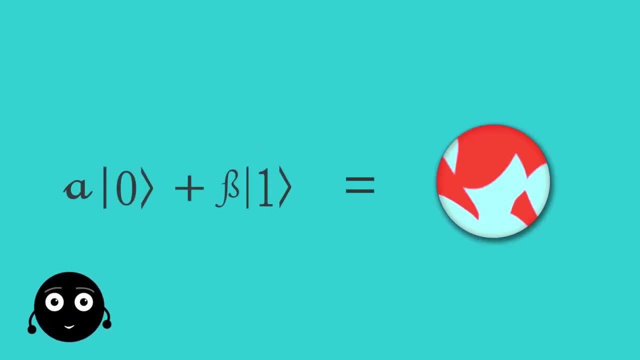 It is perfectly legal to have a linear combination of these two states. This phenomenon is called quantum superposition. The numbers alpha and beta are, in general, complex numbers. The special states ket 0 and ket 1 are known as computational basis states and form an orthonormal basis for this vector space. 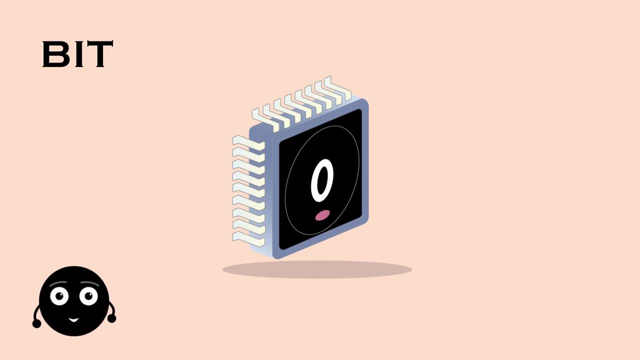 Let's now explore the fundamental difference between a bit and a qubit. It is always possible to examine a bit to determine if it is in state 0 or 1.. Computers do this all the time when they retrieve the contents of their memory. 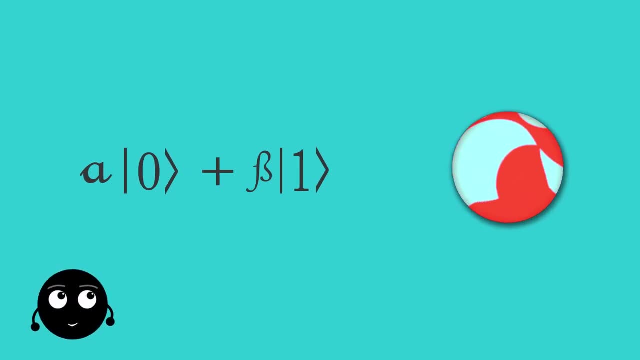 Rather. remarkably, it is not possible to examine a qubit to determine its quantum state. For learning the quantum state of a qubit, we need to learn the values of alpha and beta. However, quantum mechanics tell us that we can only acquire much more restricted information about the quantum state. 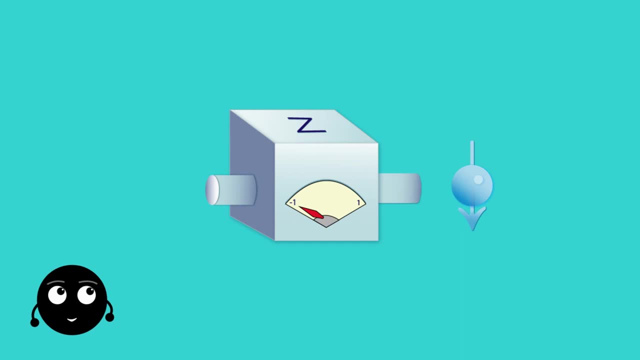 When we measure a qubit we get either the result ket 0 with probability alpha squared, or ket 1 with probability beta squared. So from a single measurement we will not be able to learn the values of both alpha and beta. 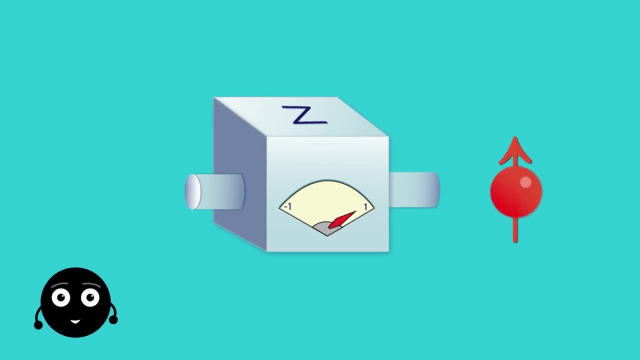 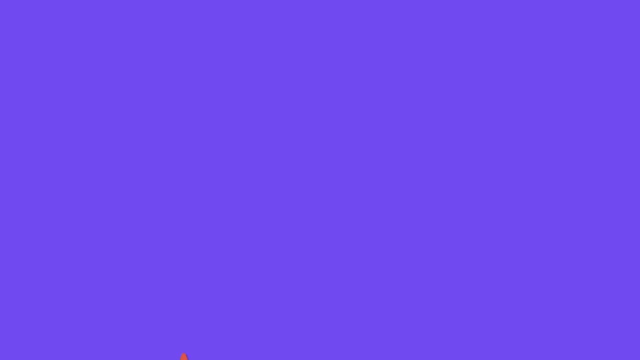 Thus, in general, a qubit state is a unit vector in a two-dimensional complex vector space and measurement collapses it into one of the bases. Qubits' ability to be in superposition states runs counter to our common sense. A classical bit is like a coin: either heads or tails up. 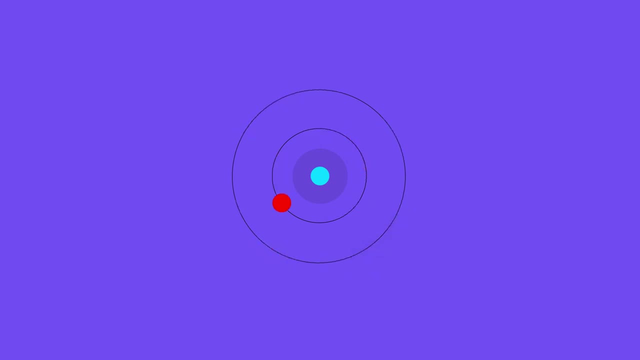 By contrast, a qubit can exist in a continuum of states between ket 0 and ket 1, until it is observed. Let us emphasize again that when a qubit is measured, it only ever gives 0 or 1 as the measurement result. probabilistically, For example, a qubit can be in the state which 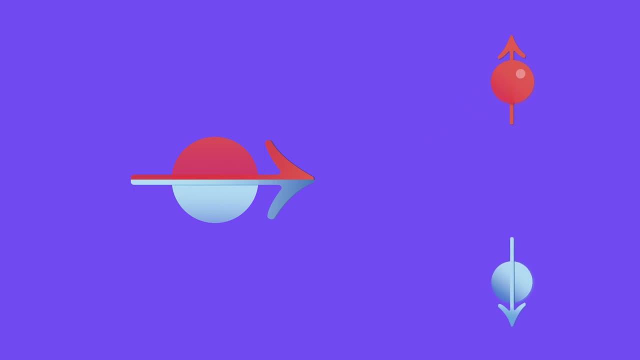 when measured, gives the result 0- 50% of the time and the result 1, 50% of the time. This state, which is in an equal superposition of ket 0 and ket 1, is quite an important quantum state. 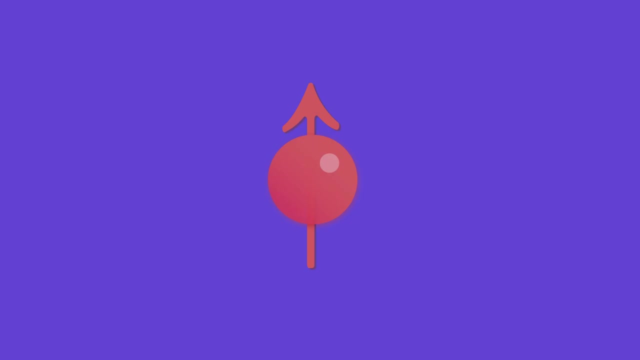 and is sometimes denoted by ket plus. Although qubits seem strange, they are in fact real. experiments extensively validate their existence and behavior, and they can be realized using a wide range of physical systems. In order to get a sense of how a qubit can be realized, let's see some of the ways it can occur. 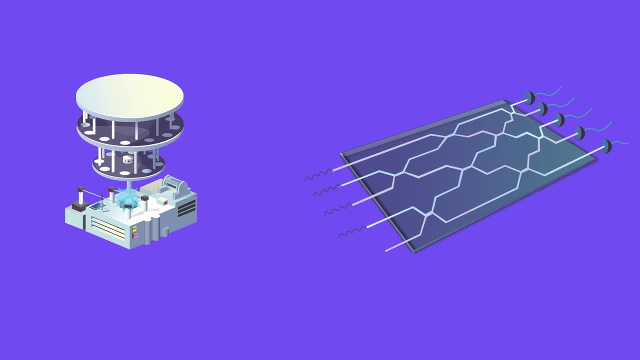 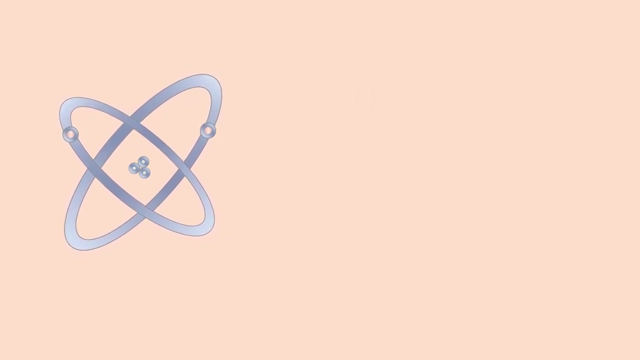 As the two different polarizations of a photon, as the alignment of a nuclear spin in a uniform magnetic field, as two states of an electron orbiting a single atom. In the atom model, the electron can exist in either the so-called ground or excited states, which we'll refer to as ket 0 and ket 1 respectively. 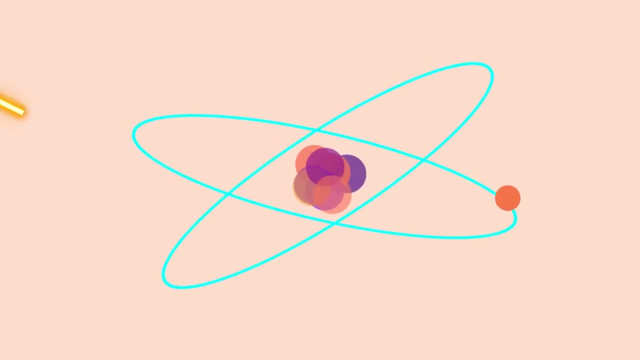 By shining light on the atom, with appropriate energy and for an appropriate length of time, it is possible to move the electron from the ket 0 state to the ket 1 state and vice versa, But, more interestingly, by reducing the time we shine the light. 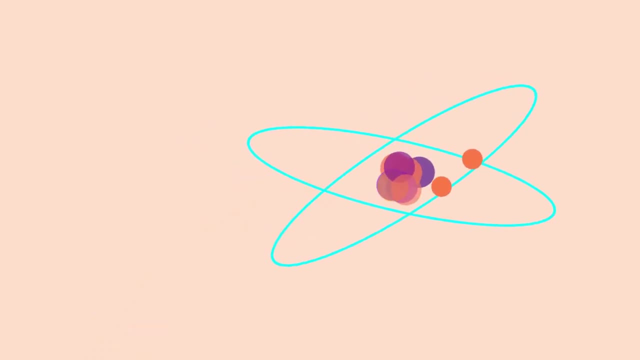 an electron, initially in the state of ket 0, can be moved halfway between ket 0 and ket 1 into the ket plus state. Historically, a great deal of attention has been given to the meaning or interpretation that might be attached to superposition states. 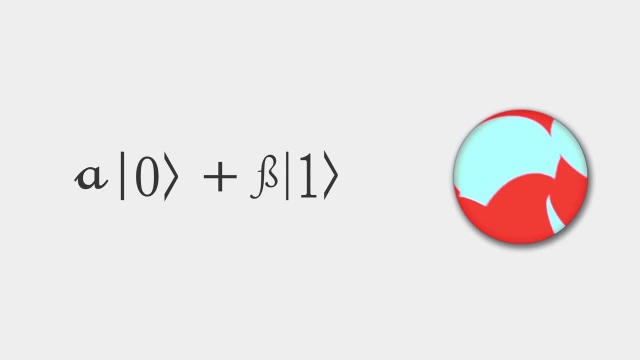 and to the inherently probabilistic nature of observations on quantum systems. However, for almost all practical purposes related to quantum information processing, it is not necessary to concern with such discussions How much information is represented by a qubit. Paradoxically, we can do infinite binary expansion. 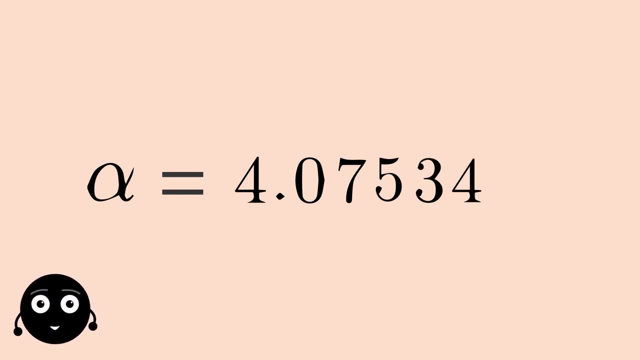 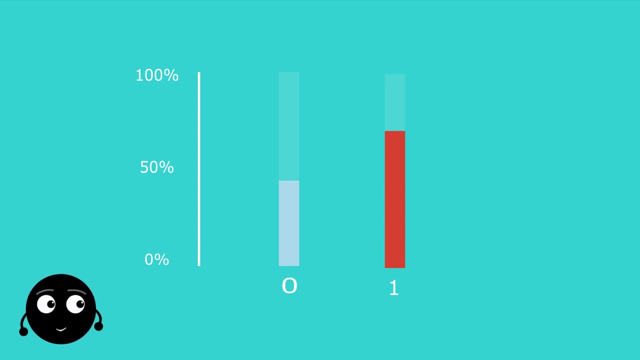 of values- alpha and beta- so in principle it could store infinite information. However, this conclusion turns out to be misleading because of the behavior of a qubit when observed. Recall that the measurement of a qubit will give only either 0 or 1.. Furthermore, measurement changes. 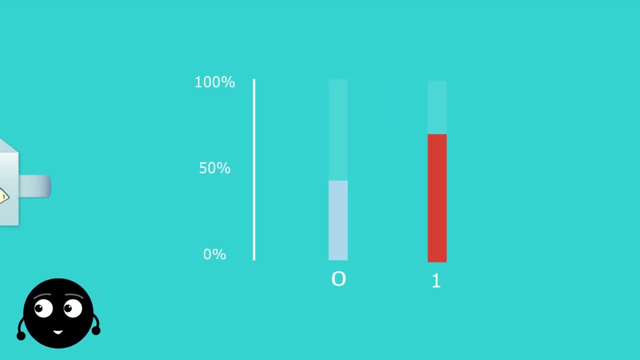 the state of a qubit, collapsing it from its superposition of ket 0 and ket 1 to the specific state consistent with the measurement result. For example, if the measurement of ket plus gives 0,, then the state of the qubit after measurement will be ket 0.. Why does this type of collapse occur?